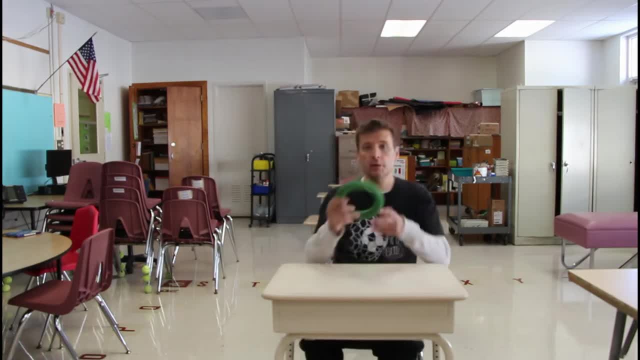 play with your class, right, And it's basically a relay. So what I would do is I would take the deck ring and you can use anything. I'm going to pass it over to the person that's behind me and then I'm going to take their place in that seat and they're going to do the same thing. 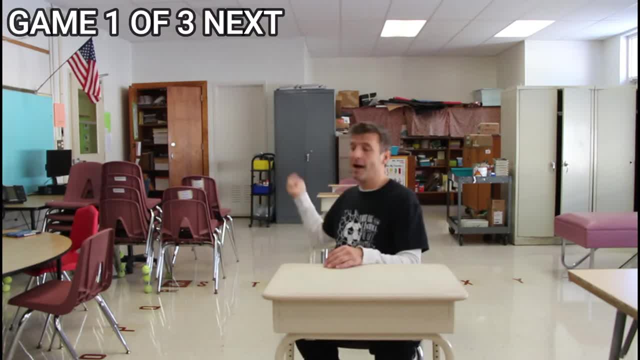 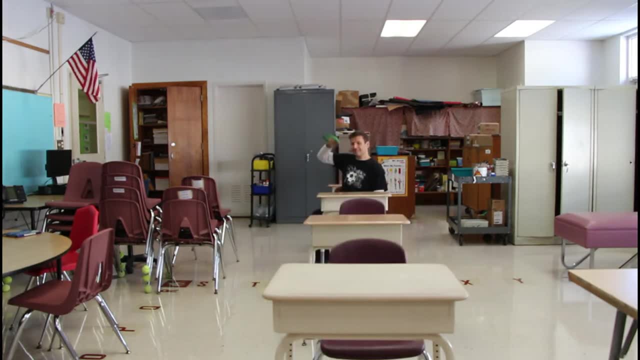 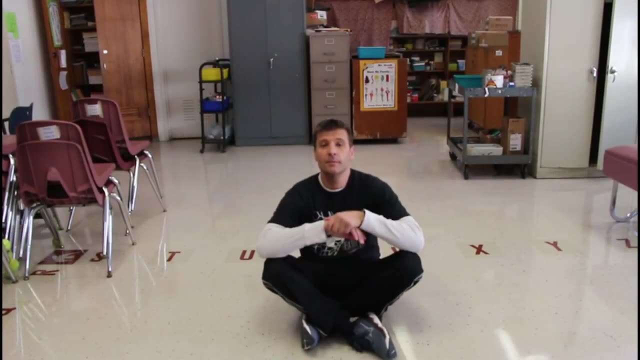 And then, when it gets to the last person, they're going to run to the front and the process is going to keep going until you get back to your original seat. Okay, this next game is called Buzz. It's a math game. Now, if you want to incorporate exercise, 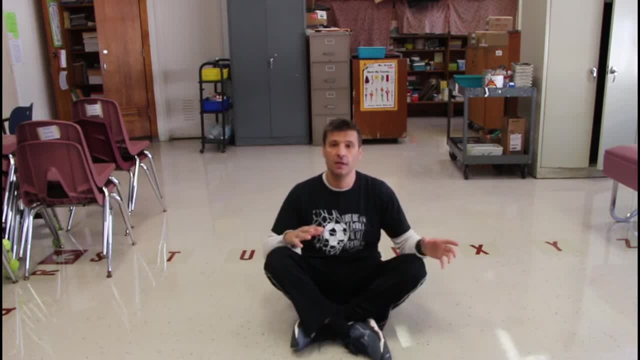 if a player gets out, you can do that, or you can have stations set up when somebody gets out until another round starts. okay, But basically in this game I find that seven is one of the best numbers to use, right? So you're going to sit the kids in a circle. they could be in a chair on the floor. 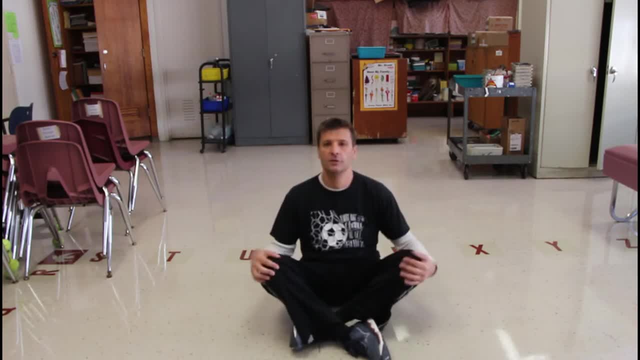 whatever, all right, And this is a great classroom game. or if you're kicked out of your gym, this is a great game, okay. So basically, what you're going to do is the first person. you can go counterclockwise. clockwise doesn't matter, but the first person is going to say one. 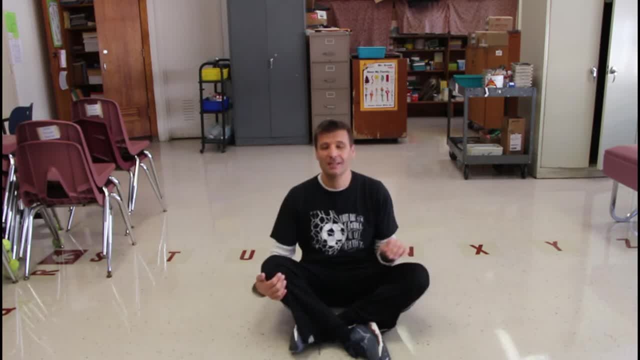 then the next person says two, next person three and so on. Anytime you get to a seven, something that has a seven in it, like 17,, or anything that is a multiple of seven. you know, seven times three is 21.. So anytime you get to any of those numbers, you have to say buzz. 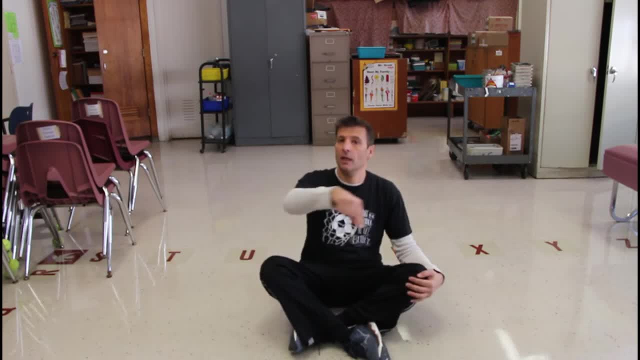 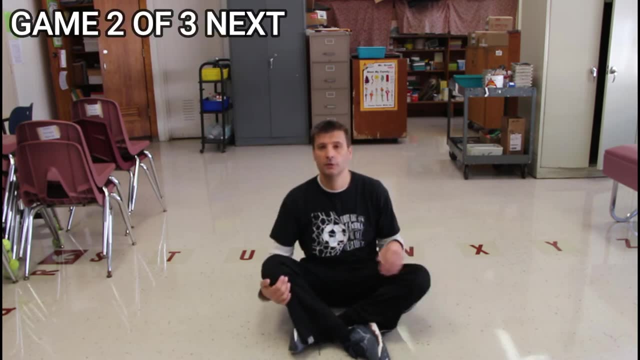 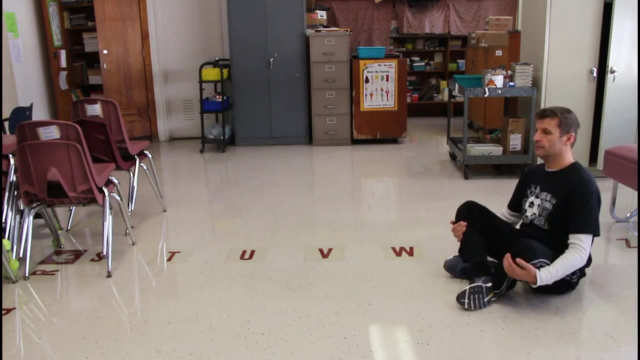 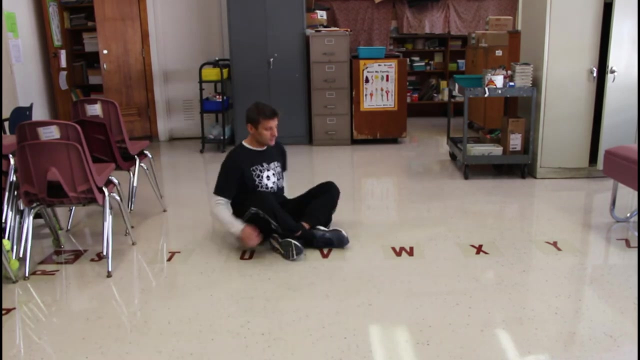 and then it changes direction. So if it was going clockwise, and then it gets to seven and that person says buzz, it now goes counterclockwise and you go to eight, One, two, three, four, five, six, buzz, eight, nine, 10,, 11,, 12,, 13,, buzz, 15,, 16,, buzz 18.. 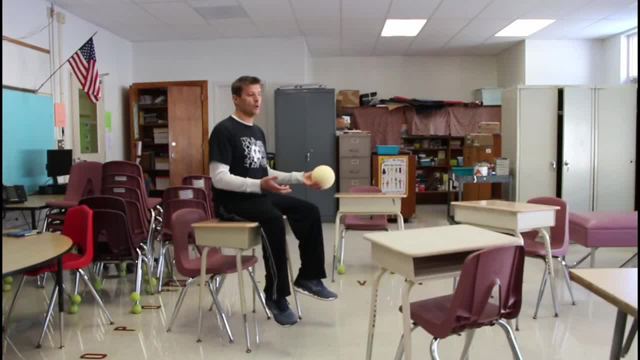 Okay, so this next game is called silent ball. I'm only using four tables to demonstrate, but you can use the entire class to do it. I have the kids set up to make it a circle and I have the kids put the desks back where they were and before you know. 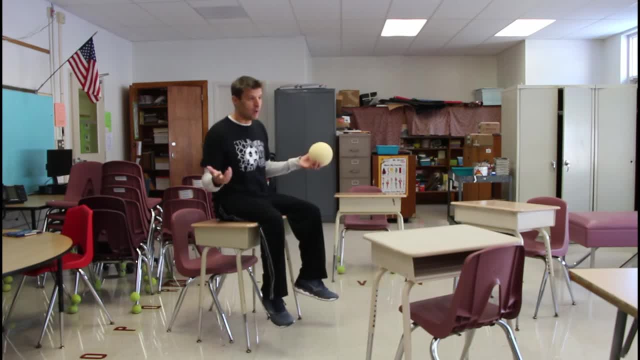 it. everything is the way it should be. Okay, so, with silent ball, obviously, once the game starts they have to be quiet, and then they can throw the ball to players at the other desks and the teacher, basically, can judge, you know, if it was a catchable ball that was dropped.